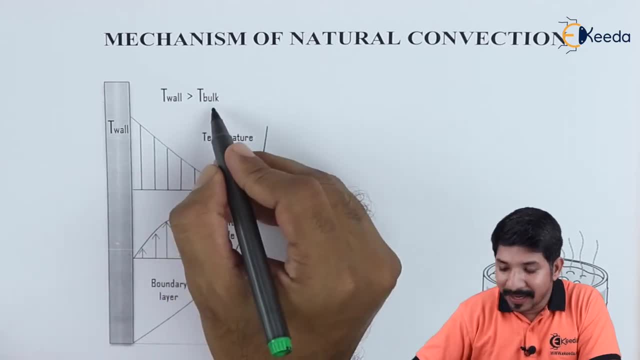 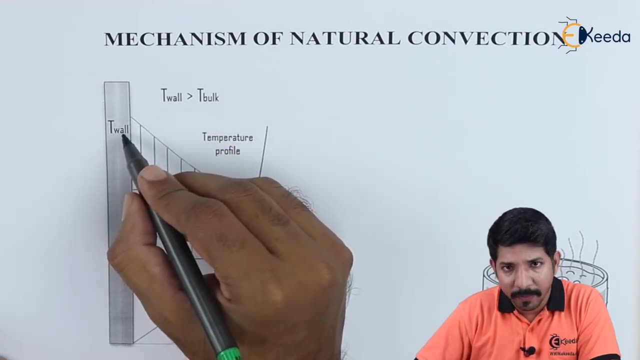 stream with a temperature equal to, let us say, T-Vol temperature. So the free stream is having a temperature of T-Vol and the wall is having a temperature of T-Vol. Now what is happening over here? In this case, as the molecules of the air will come in contact, 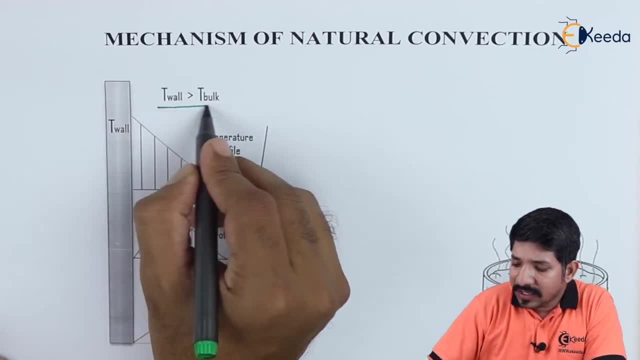 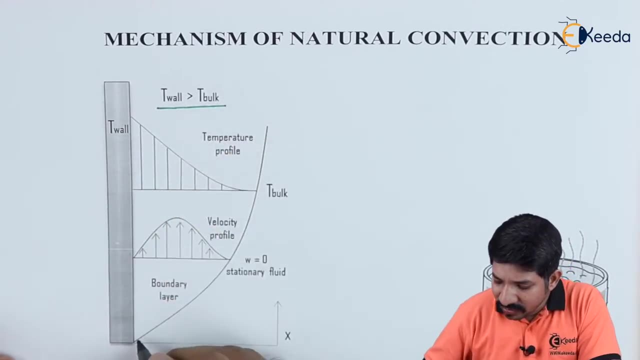 with the wall. Here we have assumed that the temperature of the wall is higher than the temperature of the bulk, That is, the air temperature. Now, as the molecules will come in contact with the wall, the temperature of the molecule will keep on increasing. 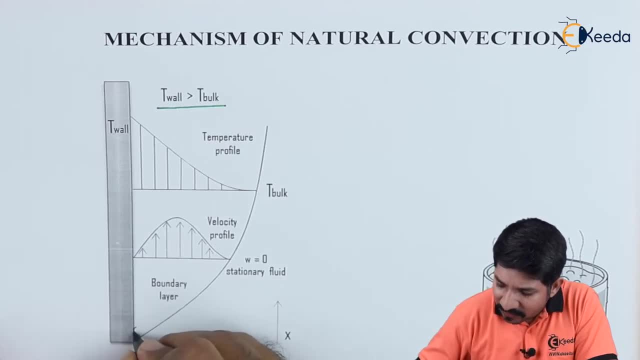 So the first molecule which is there in the contact with the wall. Now I have here exaggerated the size of molecule. You can imagine that the first molecule, the first layer of the molecule, is in contact with it. Then the second layer of the molecule will come into contactに. 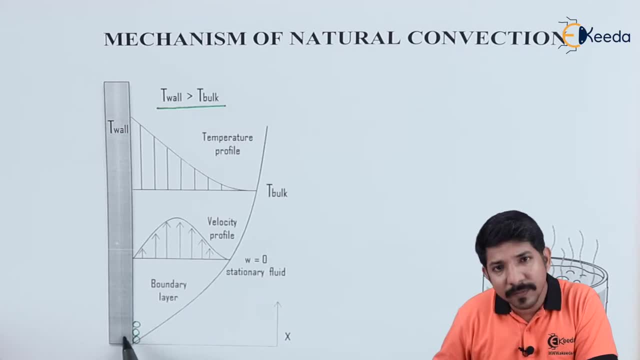 in a direct contact with the world, So the heat transfer between the two layers will be by conduction itself. Then what will happen with these molecules? Obviously, these molecules are free to move, So as the temperature of the molecule increases, the density decreases and 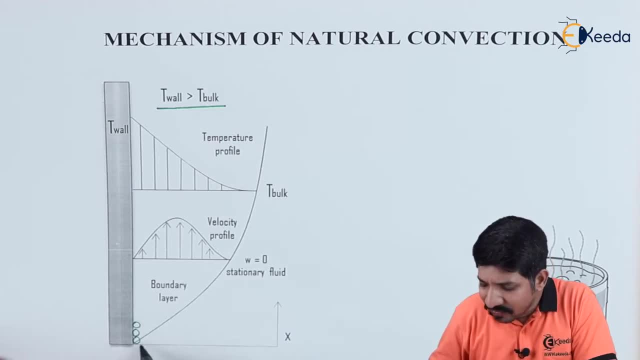 the buoyant force will come into picture. The buoyant force will obviously take them upward, So they will start moving upward, and then the void will be filled by the other molecules. The same thing will keep on happening till the current is set on. So here they have made a 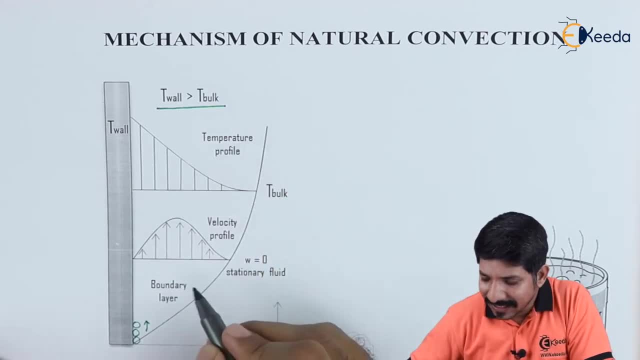 small boundary layer. Now the boundary layer is made in such a way that inside there will be some temperature gradient and outside this boundary layer the temperature of the field or the air will be the bulk temperature. So this kind of a boundary layer can only be seen in case of a 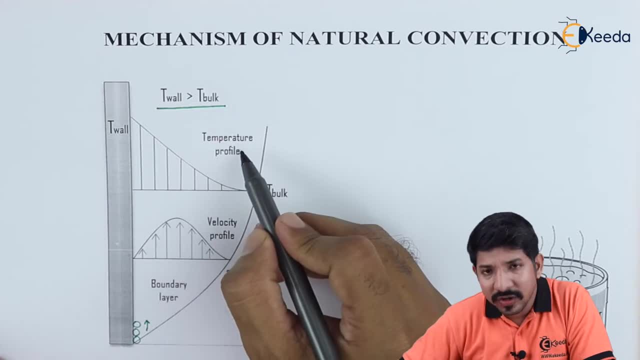 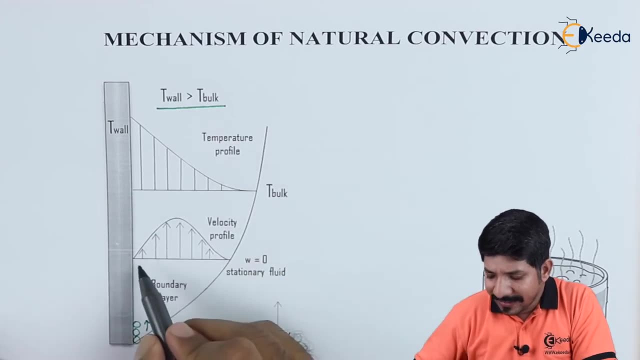 free convection. Now here they have drawn two different profiles: One is a temperature profile and the other one is a velocity profile. Obviously, in case of a velocity profile, the velocity near to the wall is zero, and so is the velocity which is outside the boundary layer, So the velocity 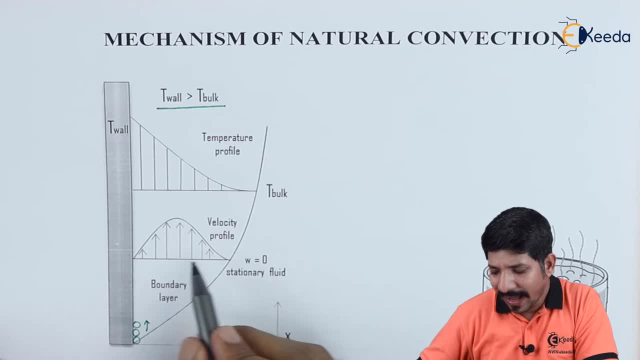 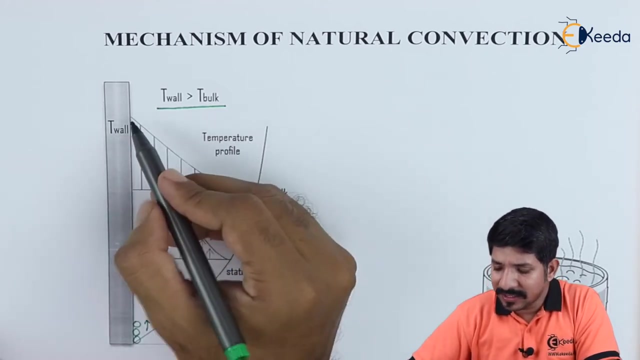 outside the boundary layer for the fluid will be zero and the velocity at the wall of the plate will also be zero. So obviously there is a parabolic nature. So at somewhere in between the velocity is the maximum. Similarly, in case of a temperature profile, the temperature at the wall is maximum and as it 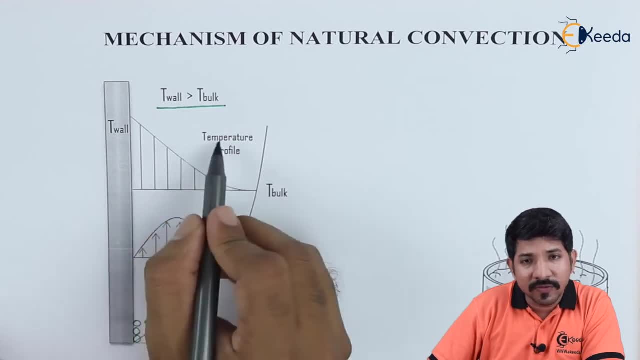 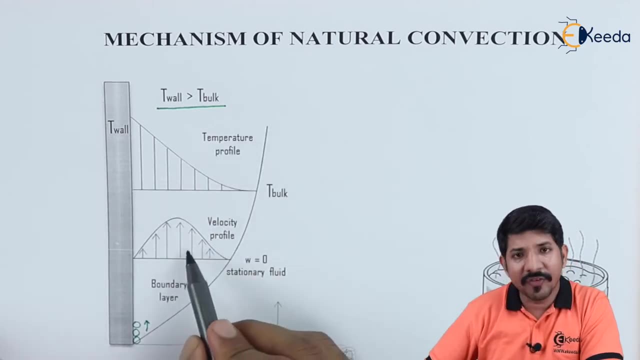 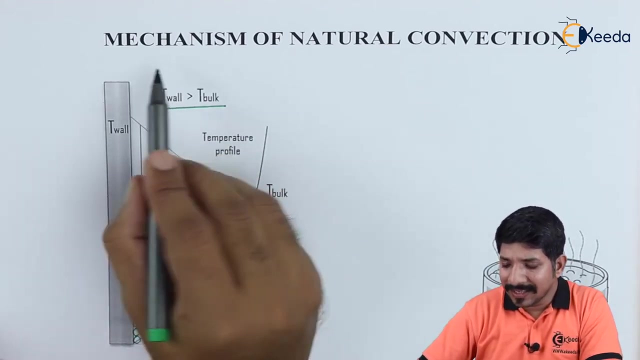 reduces or as we go further from the wall, the temperature becomes same as the bulk temperature. So obviously there exists a temperature gradient and velocity gradient, So that will make it form a boundary layer. One more way of explaining the mechanism of natural convection is by explaining 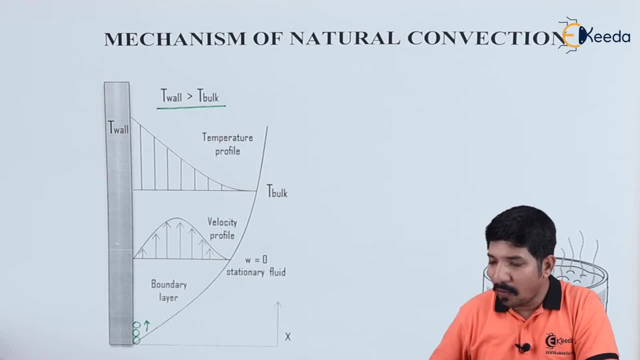 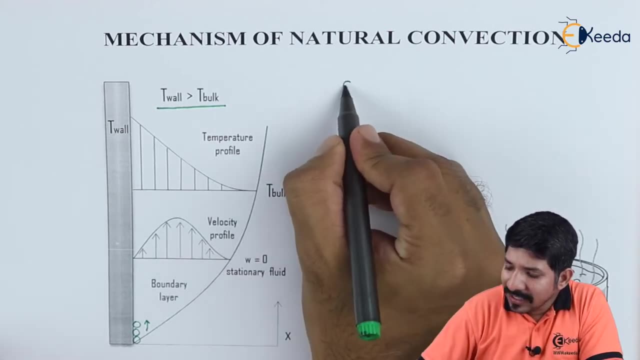 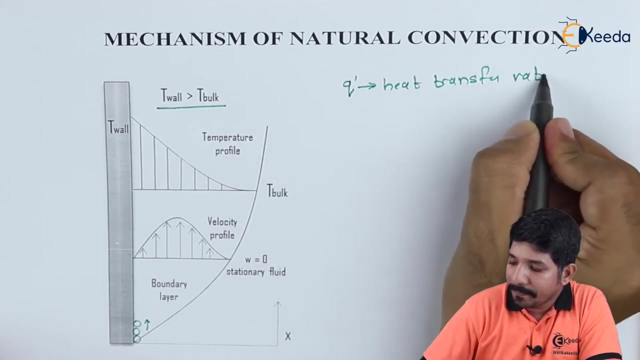 the boiling of water. Now, what is happening in case of boiling of water? How does the heat transfer takes place in case of a boiling of water? So let us say: if q- is the amount of heat transferred, q- is the amount of heat transfer rate, then how does the heat transfer rate occurs in? 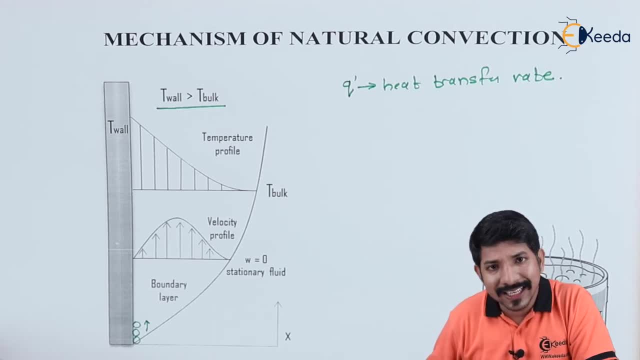 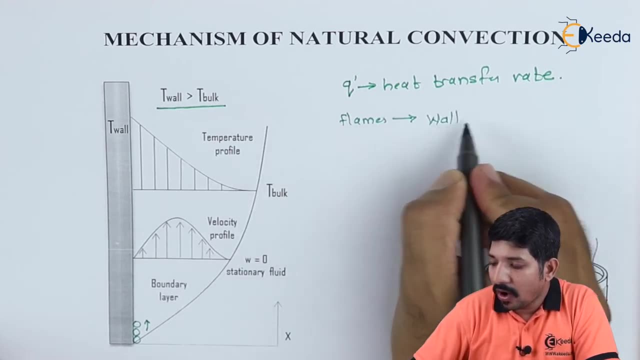 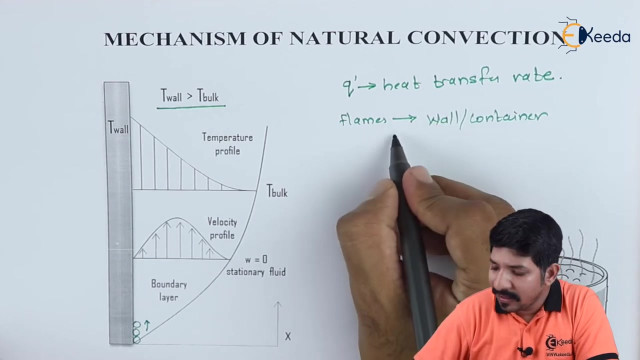 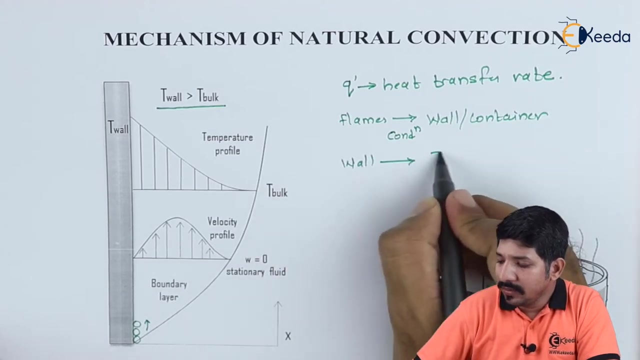 case of a boiling of water, First way is the heat is transferred from the flame to the wall or the container of the fluid. now, obviously, this heat transfer is by conduction itself, then from the wall to the first layer of water. now, again, this is done by the conduction and 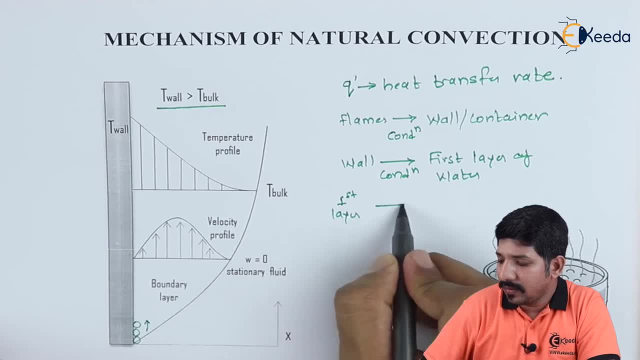 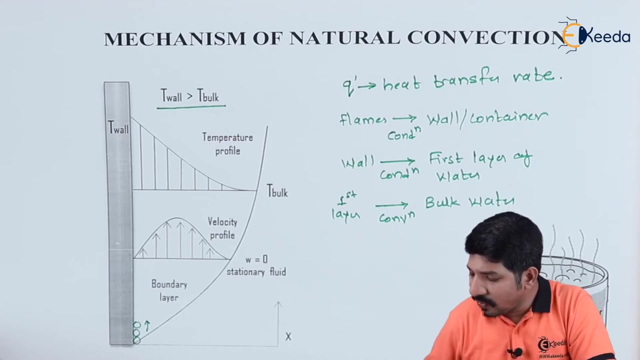 then from the first layer to the bulk water. now this is done by convection. so now this is how the boiling of the water will takes place. the heat will flow from the first layer of the solid to the first layer of the fluid. then that fluid will is free to move, so it. 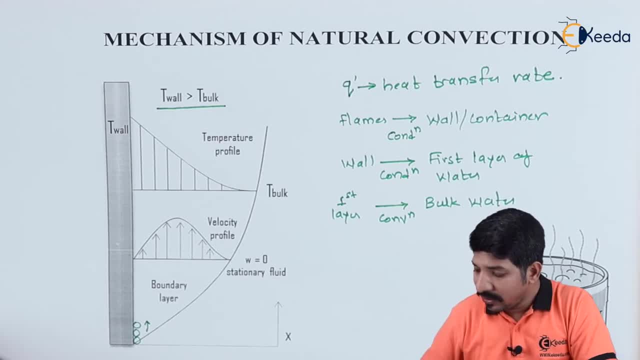 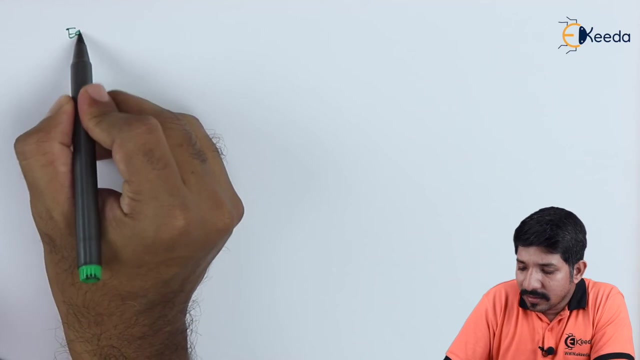 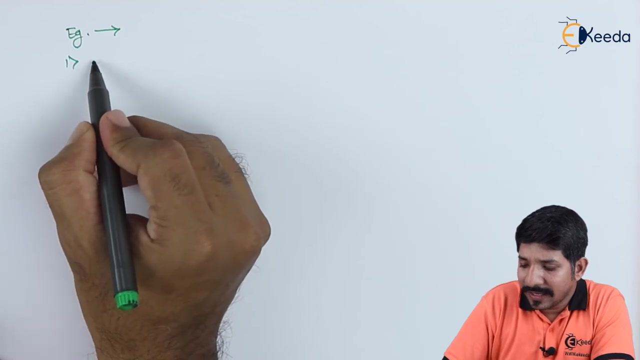 will move upward in the direction And that way the heat will transfer to the other part of the area. so this way the current will set in and then the convection, the heat transfer by convection, will occur. there are so many examples where the use of convection is there. for example, you can take the fumes. 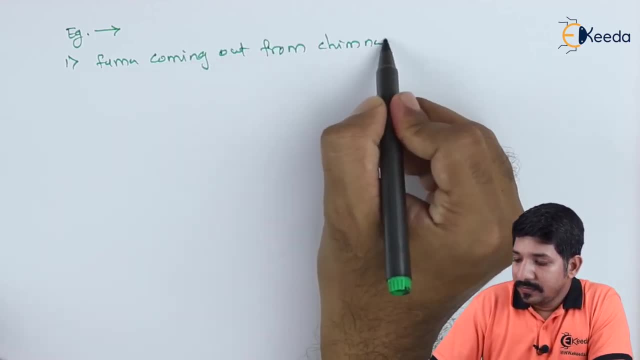 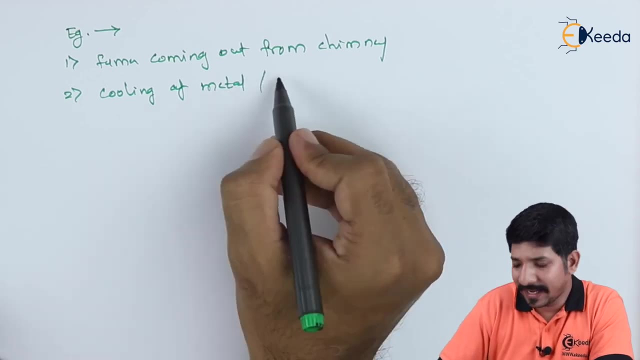 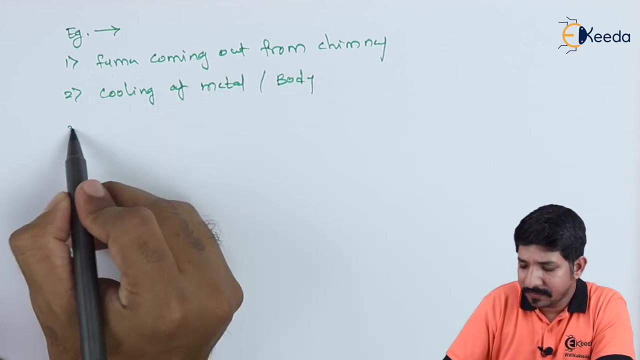 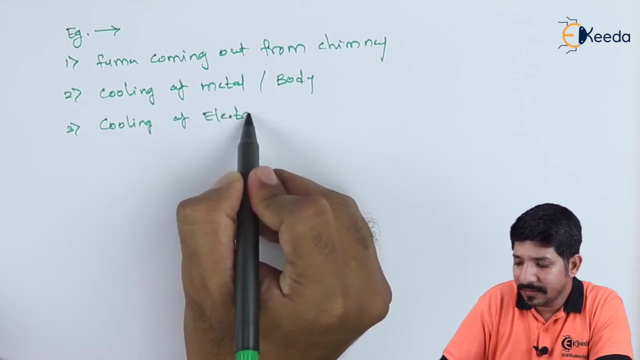 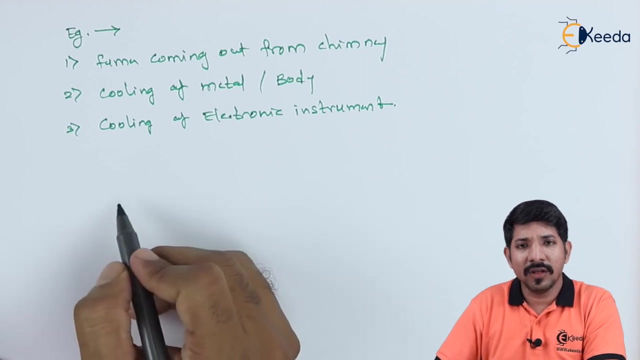 coming out from Chimneys, then the cooling of metal or for that matter, any body without force convection will require the knowledge of free convection, then the free cooling or the natural cooling of various electronic instrument. so there are so many such uses that you can see for. 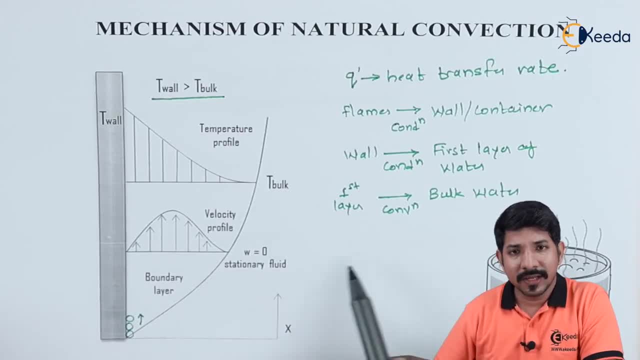 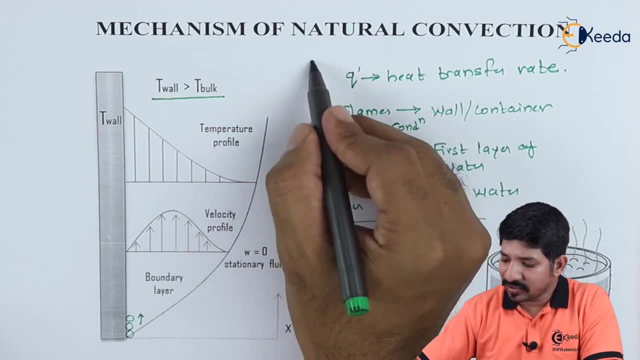 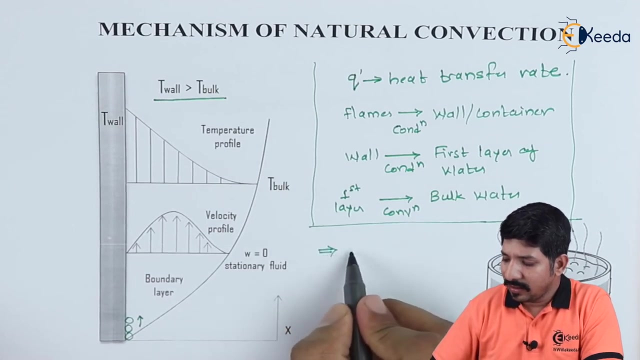 free convection itself. now, in this chapter we have tried to recognize the basic mechanism of natural convection. as we can see, or as we can illustrate from this example, that when we talk about the convection then the convection is goes with the advection plus diffusion. 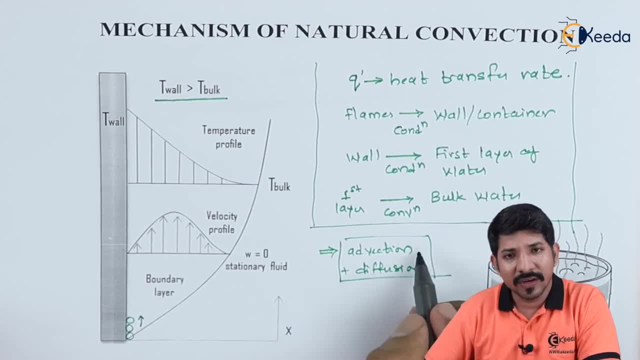 so advection is nothing, but it's a type of conduction itself, and then the convection itself, And then diffusion is the spreading of heat or the spreading of molecules in a given fluid. so altogether can be called as the convection. as we have seen, there is a molecular approach. 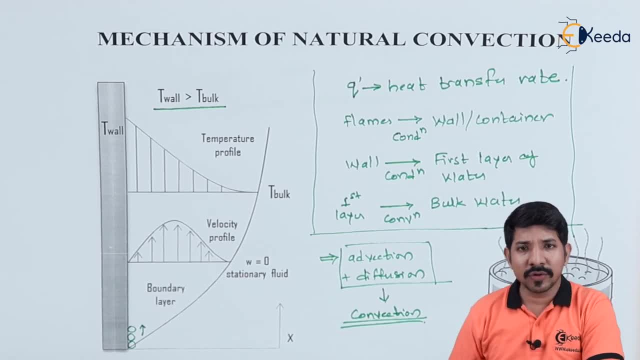 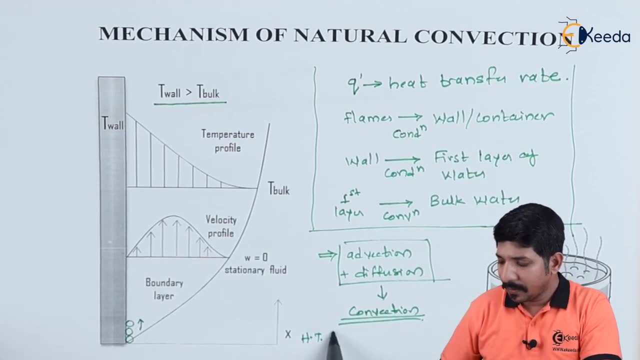 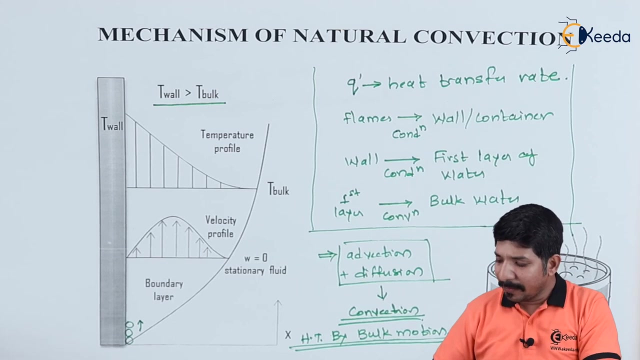 or the micro thermodynamics approach. similarly the micro thermodynamics approach can also be seen. with that I can say that convection is nothing but heat transfer by the bulk motion of fluid. if there is a bulk motion of a fluid in a given system, then we can say that the